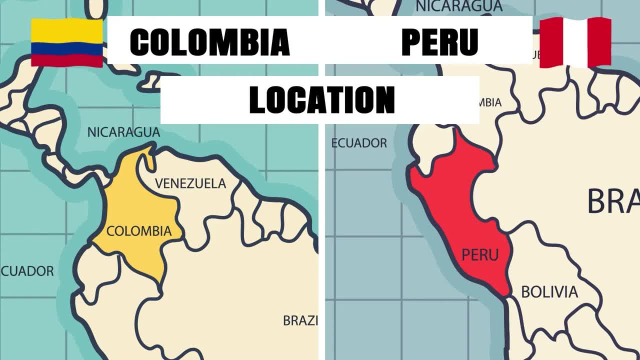 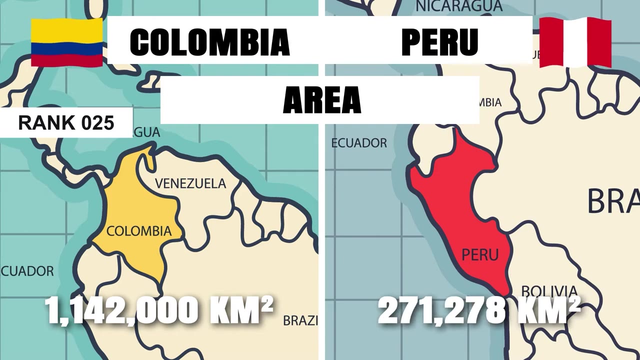 part of the continent where South America connects with Central and North America. Peru is a country in western South America. It is bordered in the north by Ecuador and Colombia Area. Colombia has an area of about 1,142,000 square kilometers. it is the 25th largest country in the world. peru has an area of about 1 million. 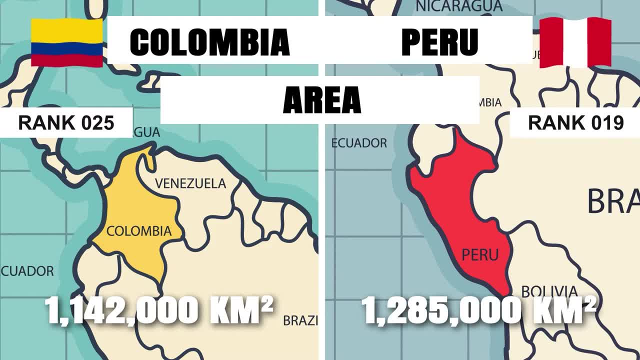 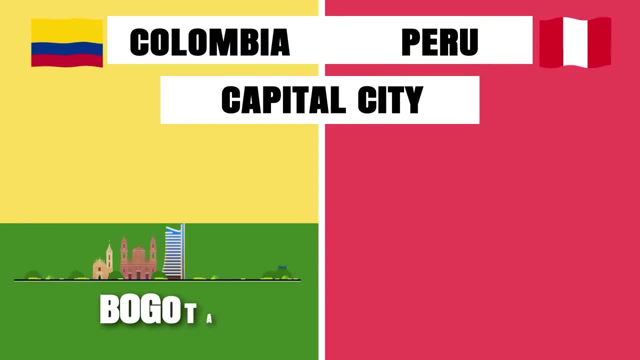 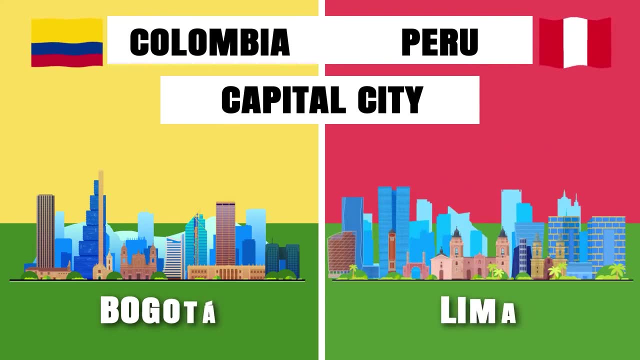 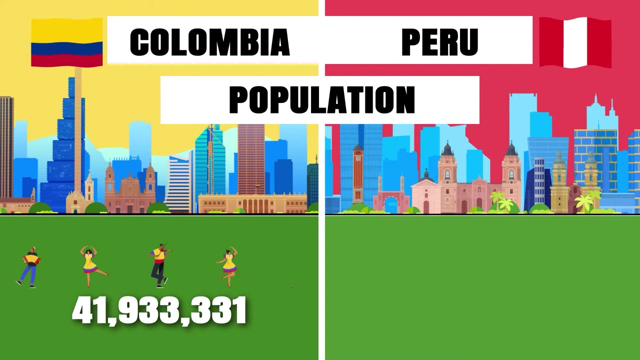 285 000 square kilometers. it is the 19th largest country in the world. capital city. the capital city and largest city of colombia is boveta. the capital city and largest city of peru is lima. population: colombia has a population of about 51 million people. it is the 28th most populated. 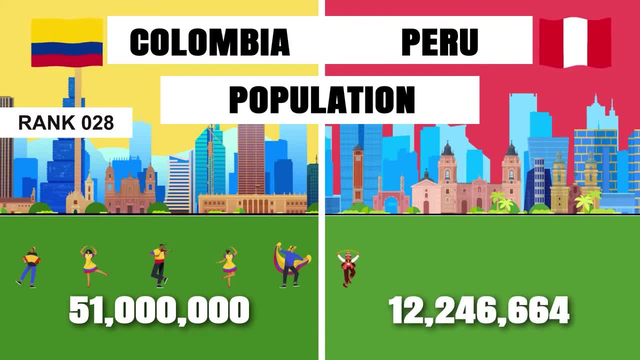 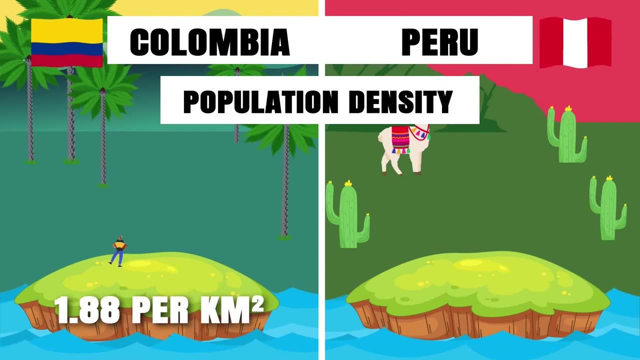 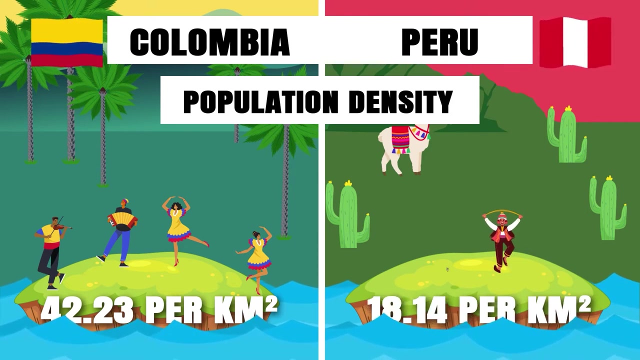 country in the world. peru has a population of about 33 million 400 000 people. it is the 42nd most populated country in the world population density. colombia has a population density about' about 42.23 people per square kilometer. peru has a population density of about 23 people per square. 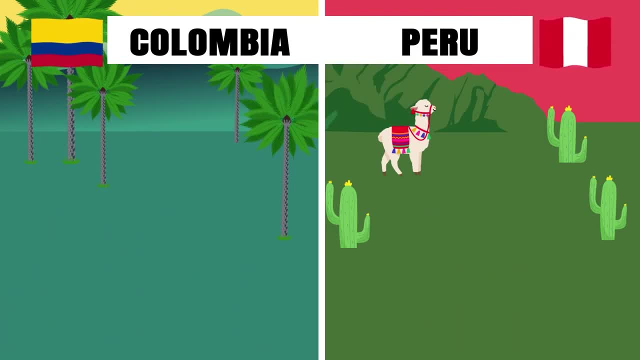 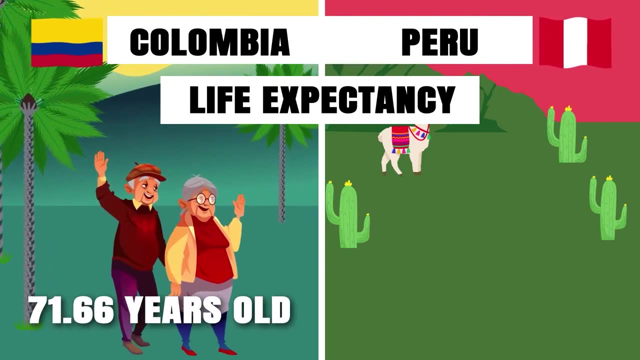 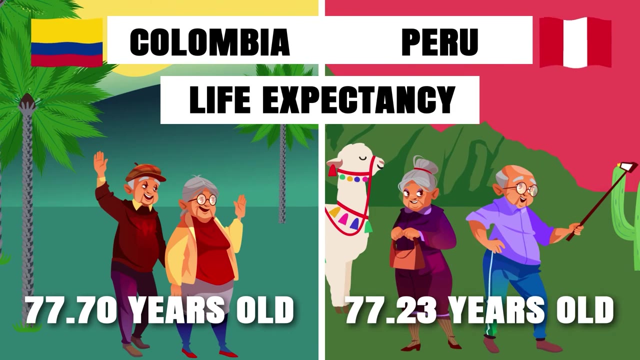 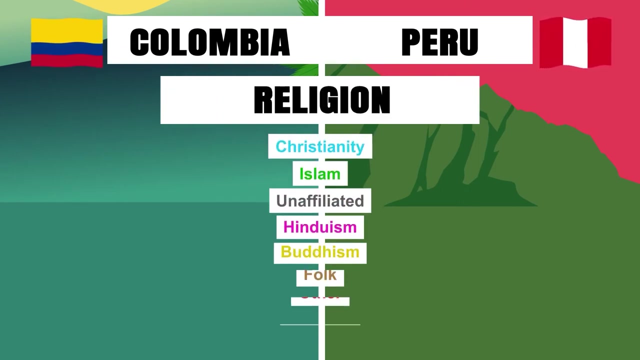 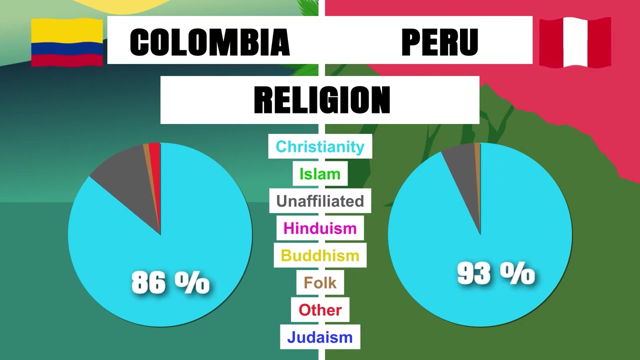 kilometer life expectancy: life expectancy for colombia in 2022 is 77.70 years. life expectancy for peru in 2022 is 77.23 years. religion: 86 percent of colombians are christian. 93 percent of peruvians are christian. 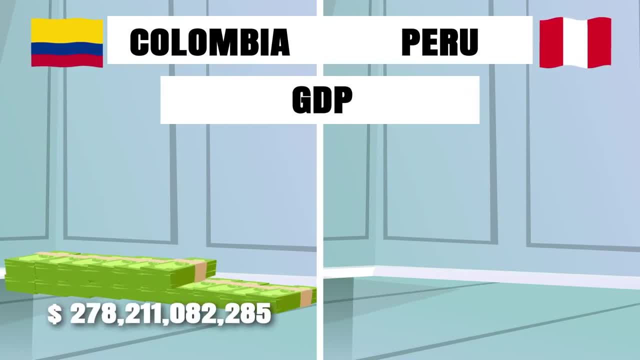 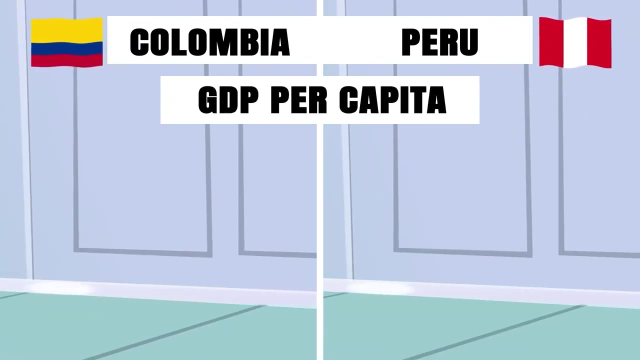 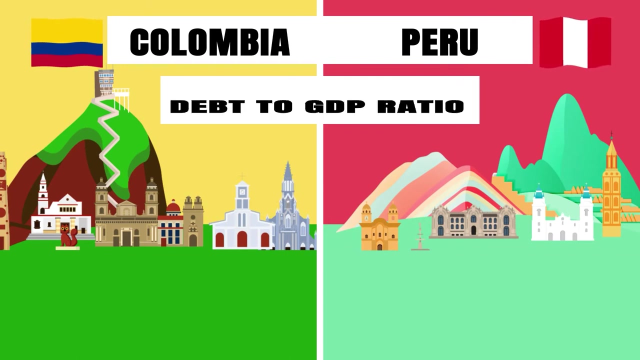 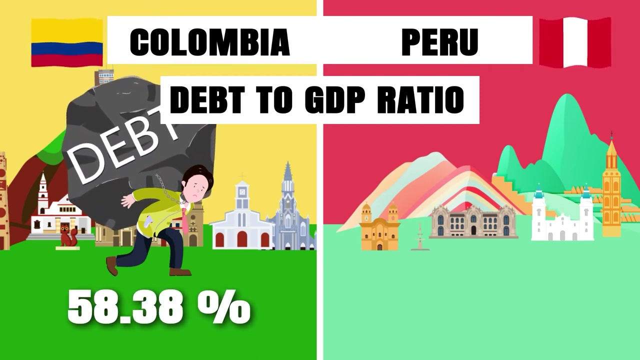 gdp: colombia has a gdp of around 343 billion us dollars. peru has a gdp of around 239 billion us dollars. gdp per capita: 6 640 us dollars. 7 000 us dollars. debt to gdp ratio: colombia's gross government debt is 61.1 of gdp. peru's gross government debt is 34.8. 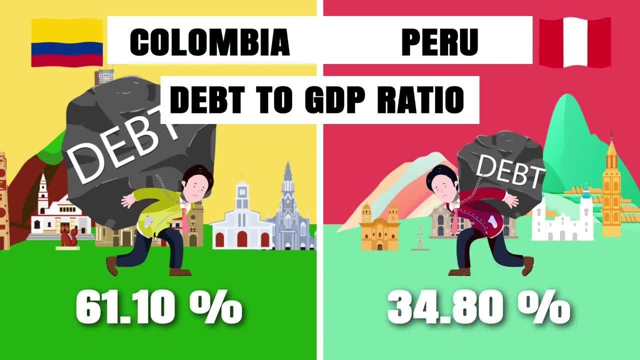 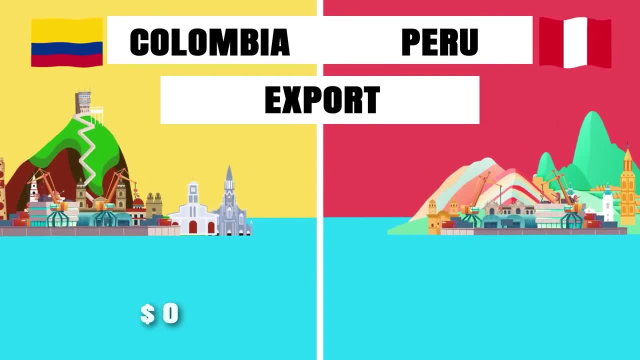 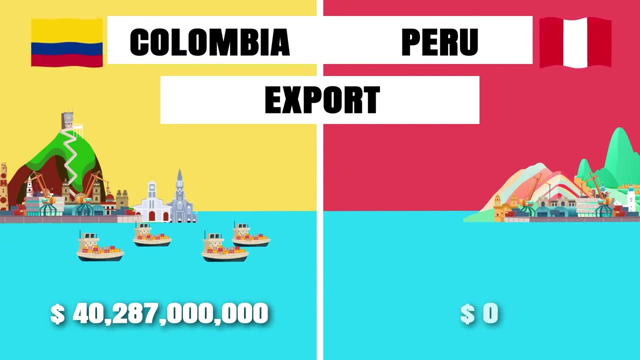 of gdp. export: colombia has a total export value of about 40 billion 287 million us dollars in 2021. peru has a total export value of about 59 billion 443 million us dollars in 2021. import: colombia has a total import value of about 61 billion 101 million us dollars in 2021. 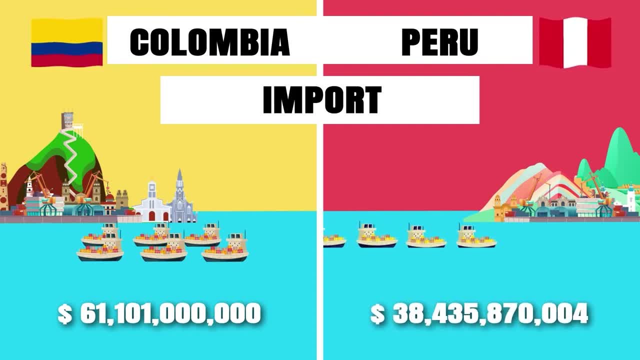 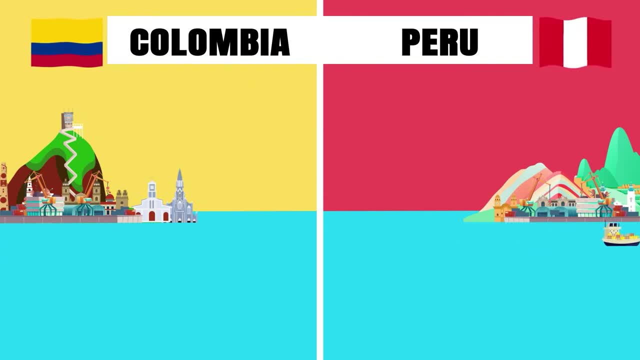 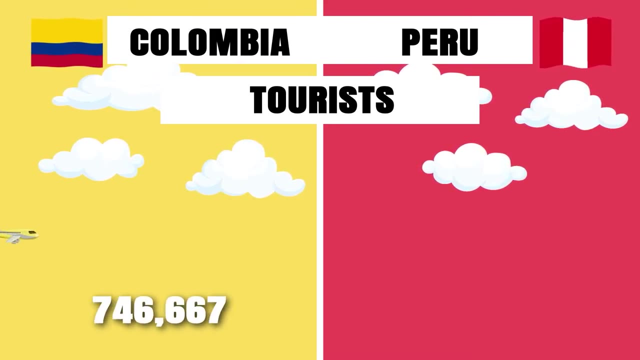 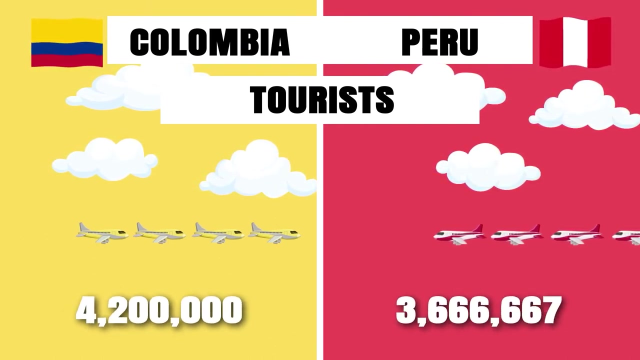 peru has a total import value of about 50 billion 871 million us dollars in 2021. peru has a total import value of about 50 billion tourists. colombia has approximately 4.2 million international tourists per year. peru has approximately 4.4 million international tourists per year. 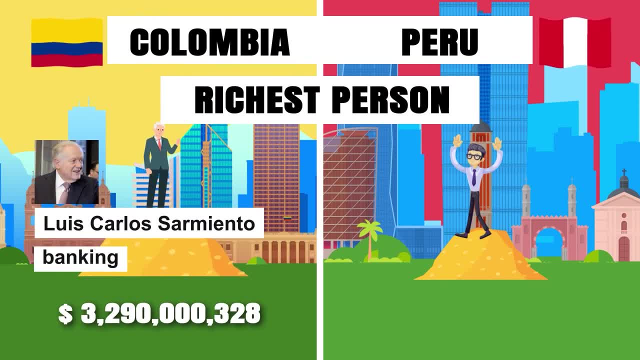 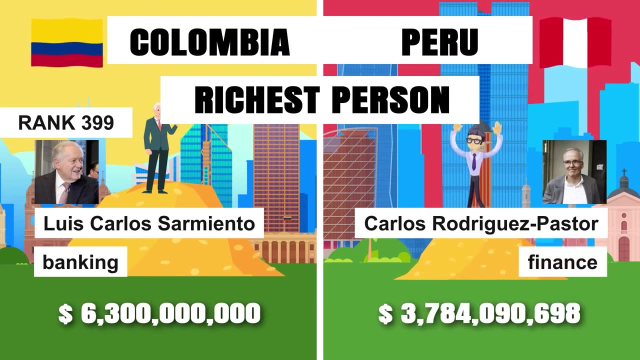 richest person. luis carlos armiento is the richest person in colombia, with a net worth of 6 billion 3 million US dollars. He was very wealthy from the construction industry and invested in banks. Carlos Rodriguez Pastor is the richest person in Peru, with a net worth of 4 billion 500 million. 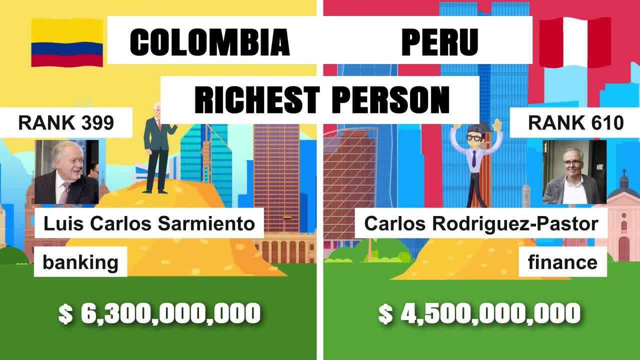 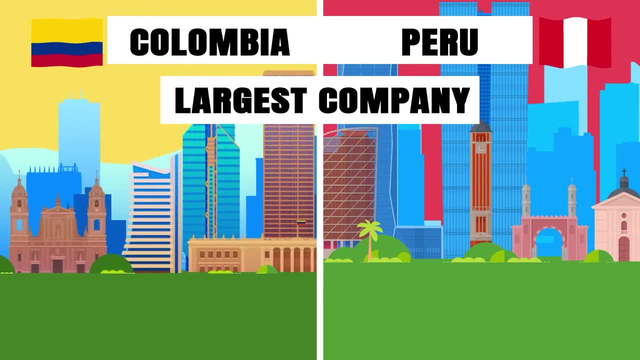 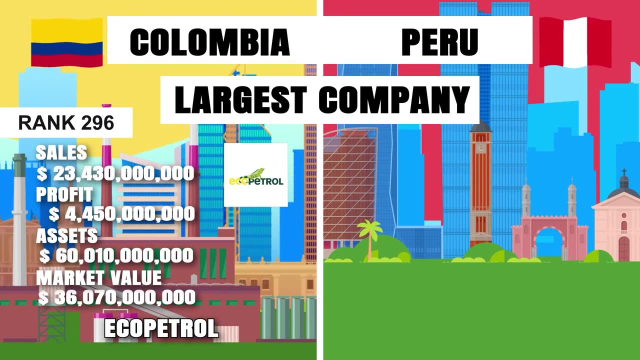 US dollars. He is a Peruvian billionaire businessman and the owner of 71% of Intergroup Financial Peruvian Banking and Retail Group Largest Company. Ecopetrol is the largest company in Colombia. It is the largest and primary petroleum company. 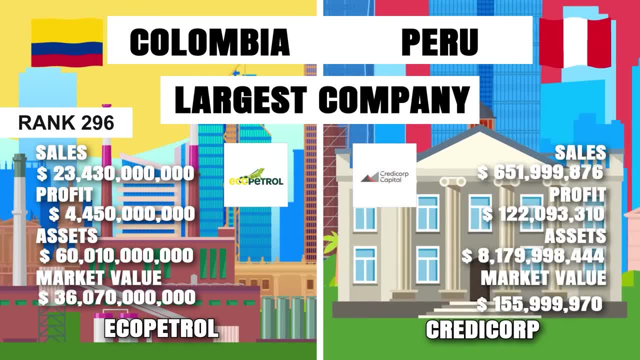 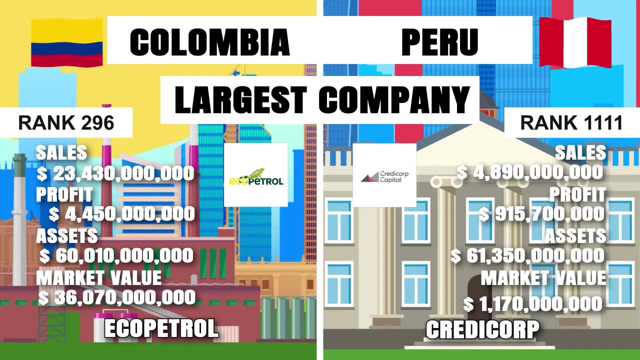 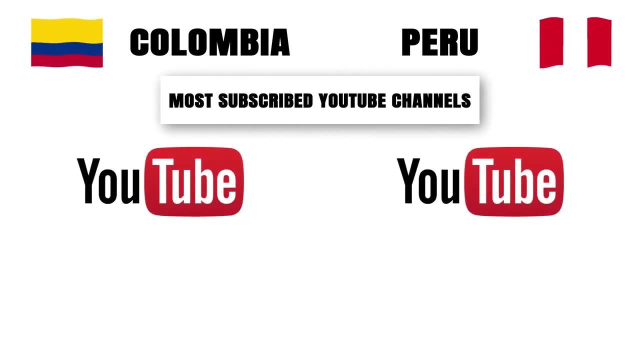 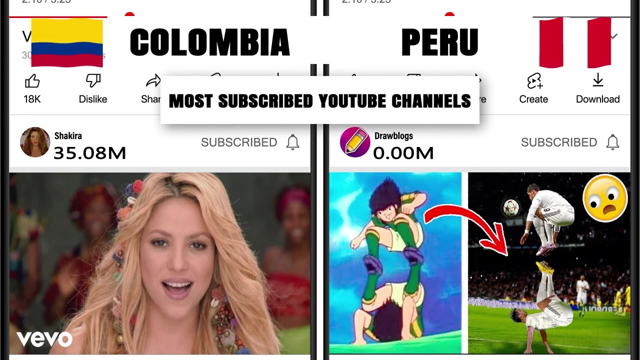 in Colombia. Credit Corp is the largest company in Peru. It is a holding company which engages in the provision of financial services. Most Subscribed YouTube Channel: Shakira is the most subscribed YouTube In Colombia, With over 38.5 million subscribers. 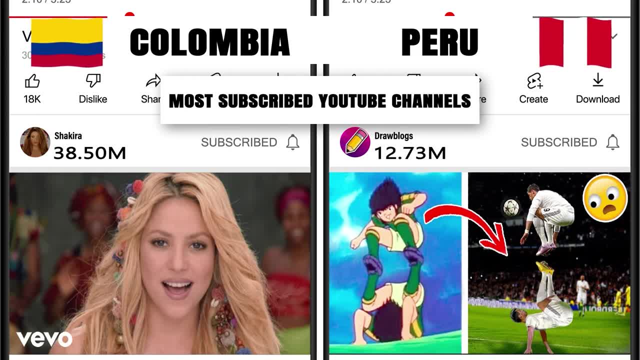 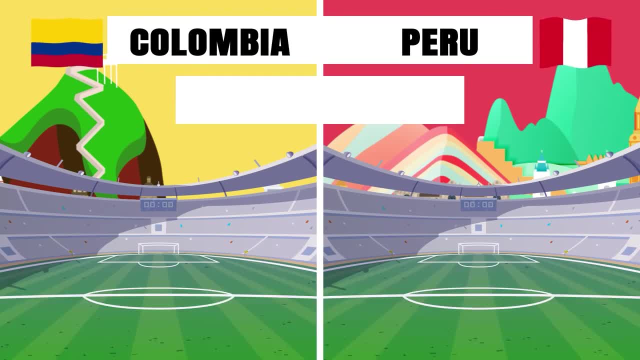 Drawblogs is the most subscribed YouTube in Peru, With over 14.5 million subscribers. Olympic Medals: Colombia won over 34 medals at the Summer Olympic Games, With 5 gold medals, 13 silver medals and 16 bronze medals.